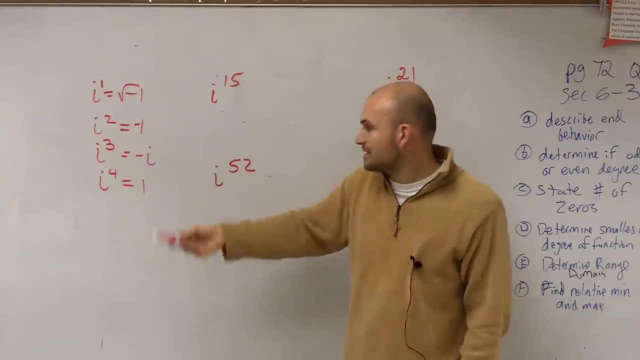 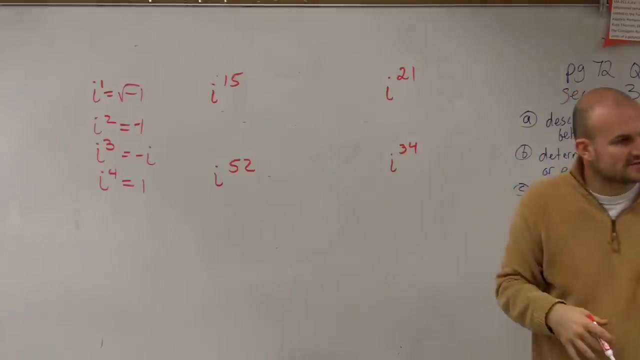 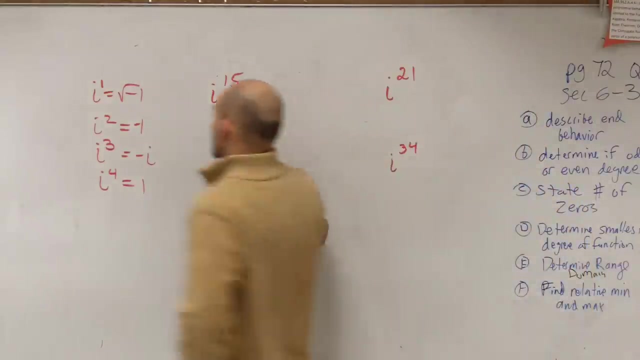 Yeah, Because think about what's I to the fourth One? If you multiply it by I, which would be I to the fifth, you're going to get back to I again, Right? Well, let's go through this. first of all, Ladies and gentlemen, you could go and write this down of I to the fifteenth as many times as you want to. So, if you wanted to, you could say: we know that I to the fourth is going to be one, So you could write this as I to the fourth. 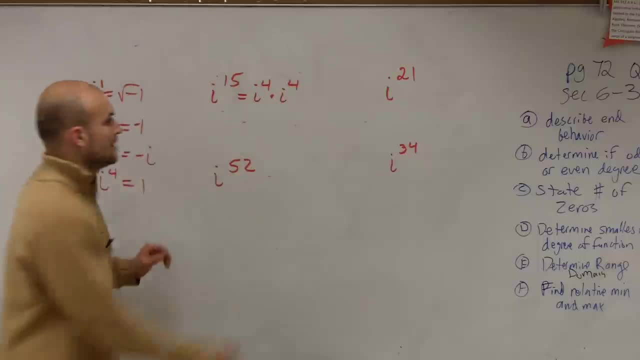 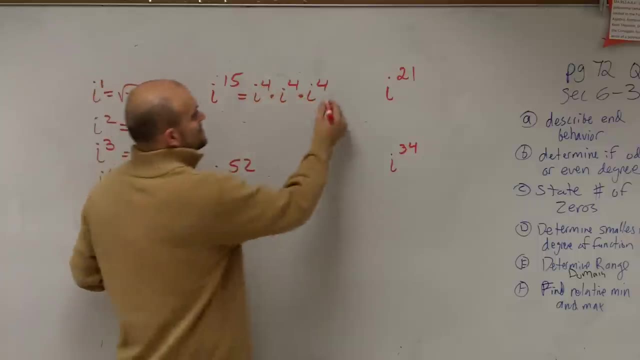 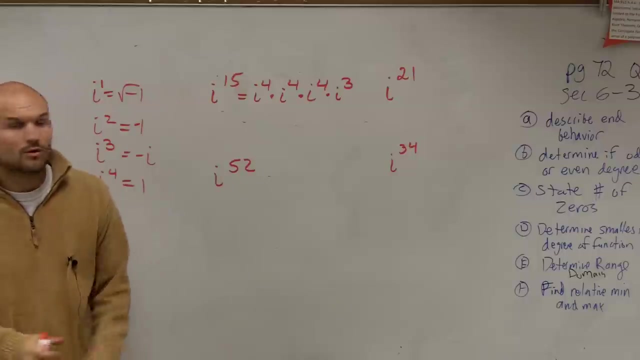 times. I to the fourth right Times. I to the fourth. So this is remember. when you multiply exponents, you add them Times. I to the third. What do you do? when you multiply exponents, You add them right. So I to the fourth times. fourth times. I to the fourth times. I cubed, is that equal to I to the fifteenth? Yeah, What's I to the fourth One. I to the fourth One. 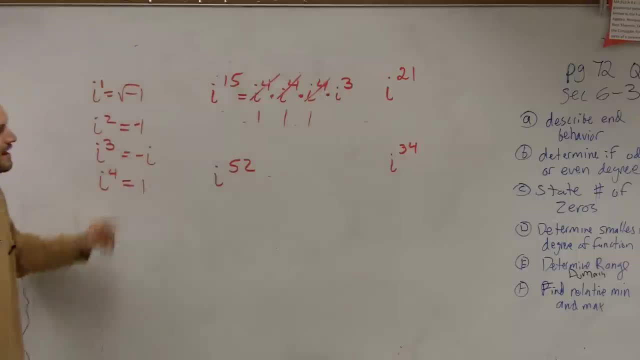 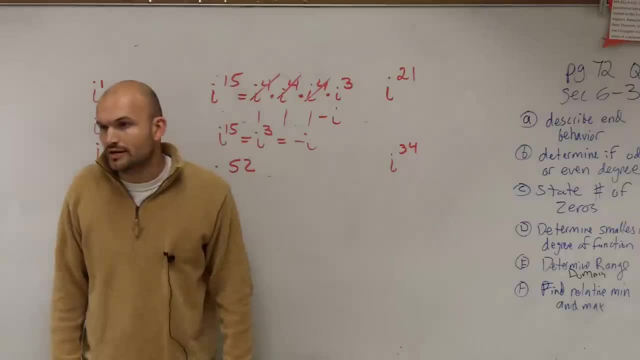 Probably not Right. So let's go and work on a shortcut. Here is a semi-shortcut. I showed you guys how to write it out, because once you get I to the fourth, we know I to the fourth is one right. 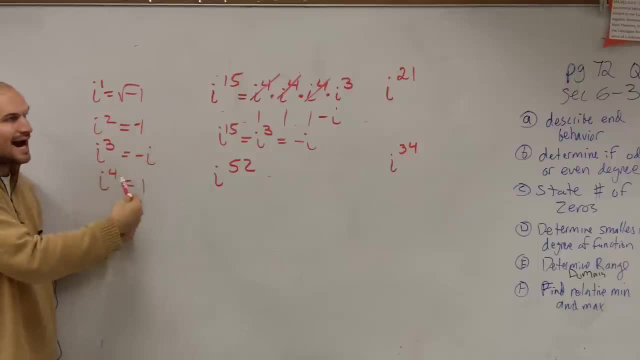 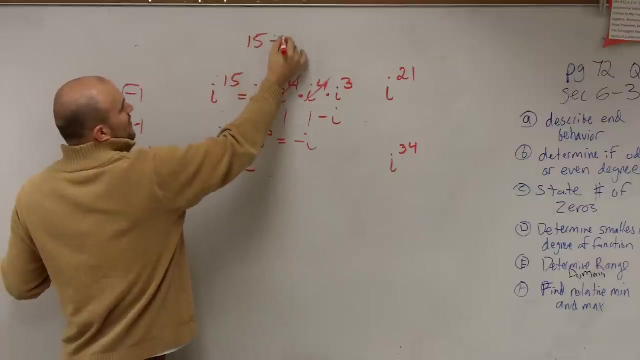 And it repeats after I to the fourth, Because I to the fifth goes back to I. Now even this, though: do we want to write I to the fourth to get up to fifty-two? What if I gave you a hundred and fifty-two? Do you want to do it that many times? No, But what you guys can do is, if I take I to the fourth rather than doing this, what I can do is I can take fifteen, all right, and divide it by four. Fifteen divided by four is what. 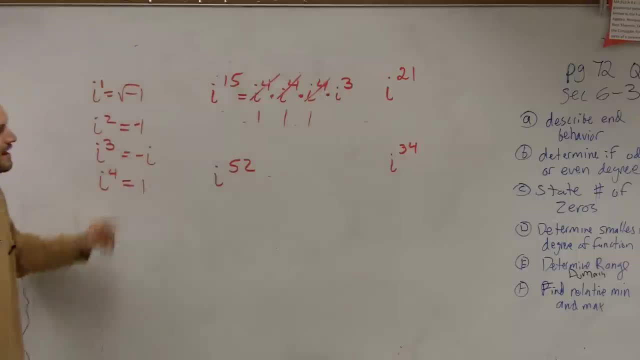 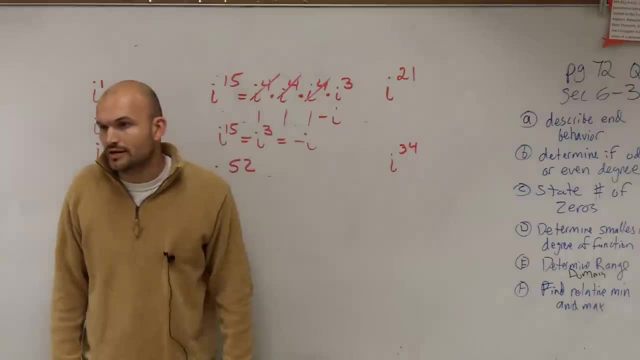 No, Probably not Right, So let's go and work on a shortcut. Here is a semi shortcut. I showed you guys how to write it out, Because once you get I to the fourth, we know I to the fourth is one Right, And it repeats after I to the fourth, Because I to the fifth goes back to I. Now, even this, though, do we want to write I? 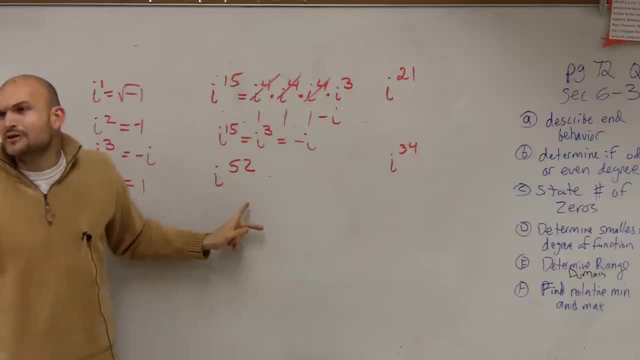 to the fourth to get up to fifty-two. What if I give you a hundred and fifty-two? Do you want to do it that many times? No, But what you guys can do is if I take I to the fourth, rather than doing this, What I can do is put that. 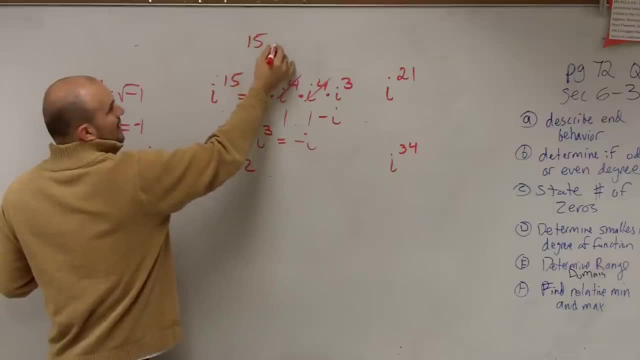 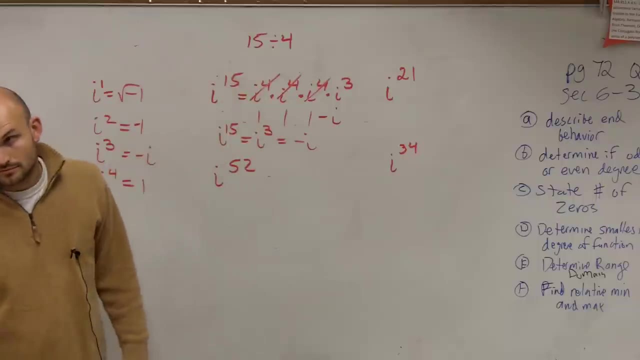 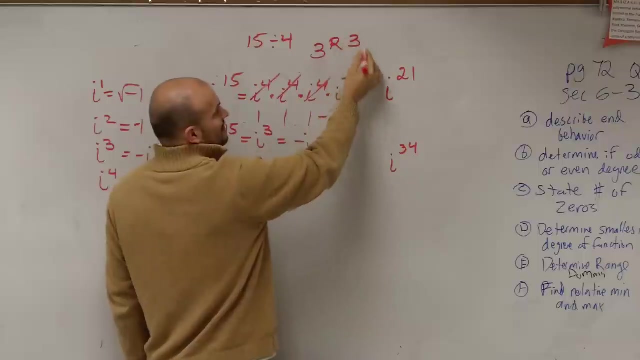 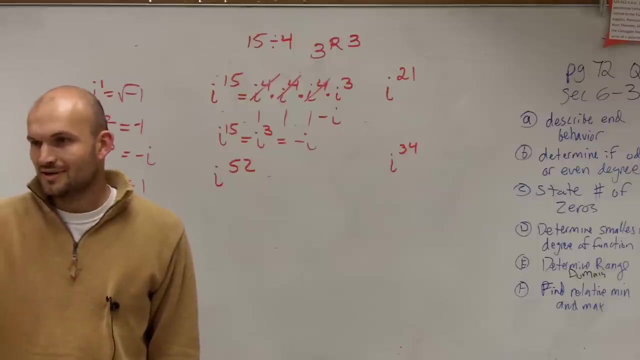 do is I can take 15 and divide it by 4.. 15 divided by 4 is what 3 with a remainder of what, 3.. 4 times 3 is 12.. You're doing the decimal right. 4 times 3 is 12.. And then. 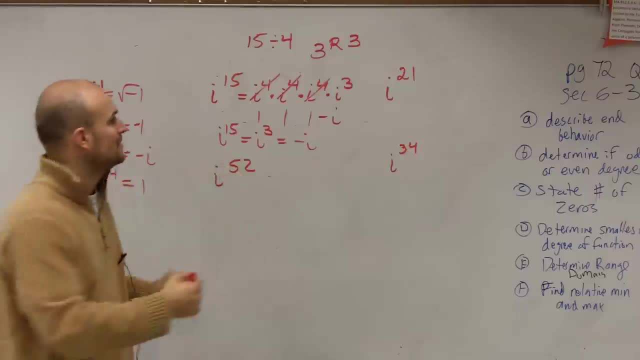 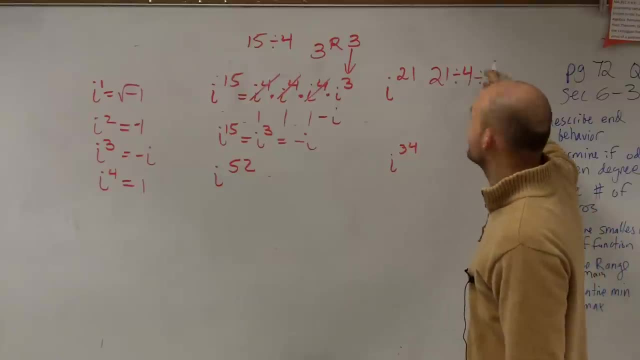 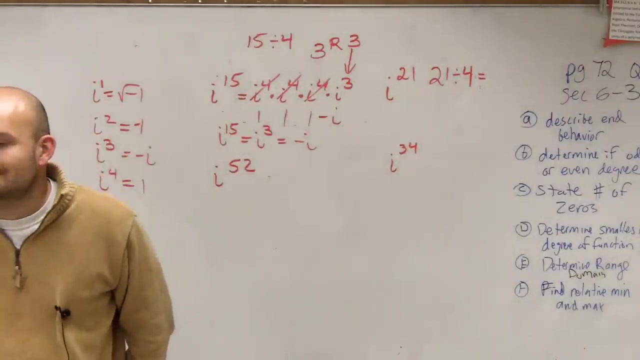 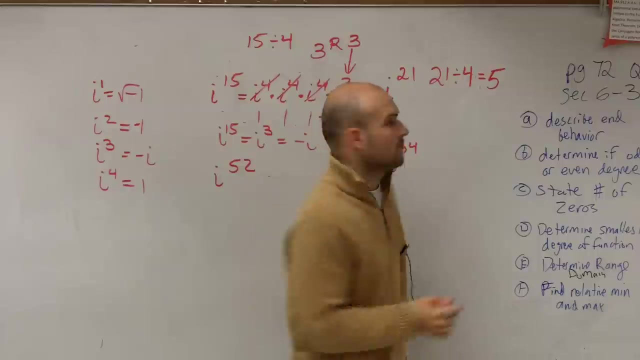 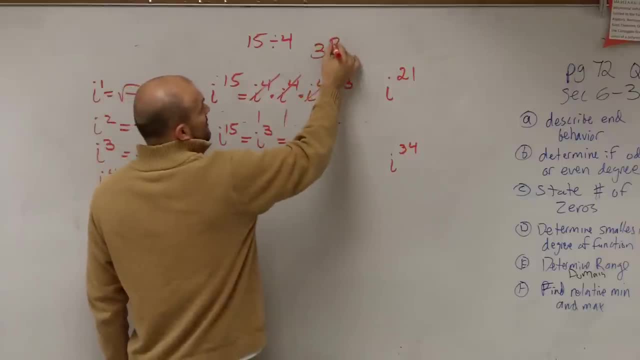 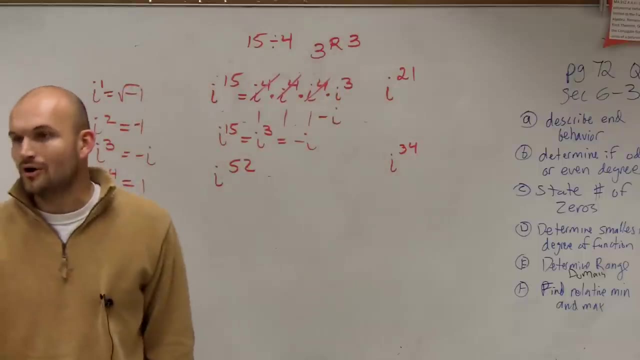 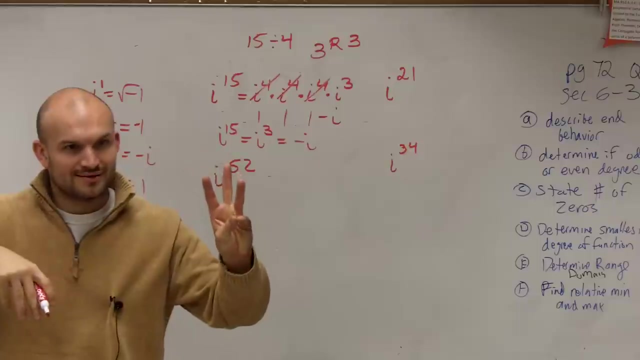 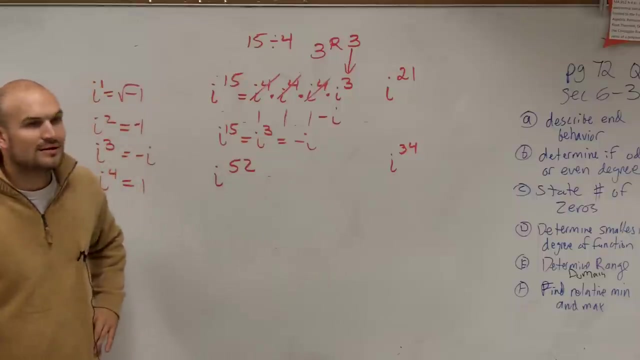 Three, Three, With a remainder of what Three. Four times three is twelve. You're doing the decimal right. Four times three is twelve, And then, to get up to fifteen, you have a remainder of what Three. Guess what That remainder is going to be: the exponent of your I, your remaining I, Okay. So let's go and do twenty-one. 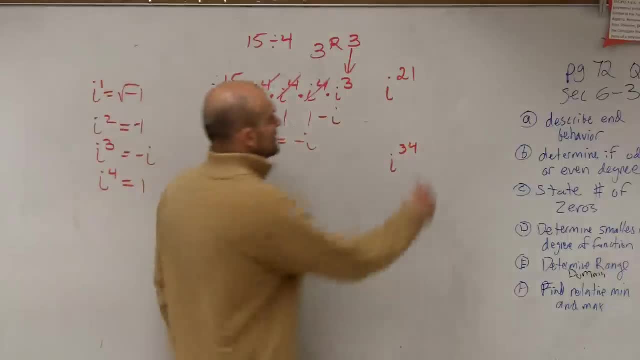 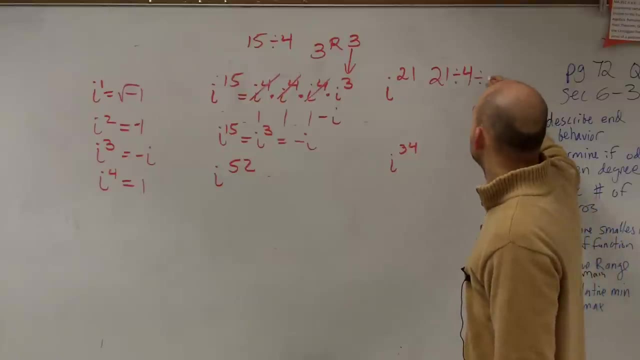 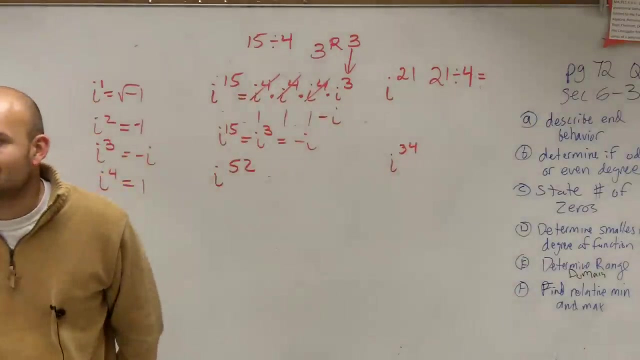 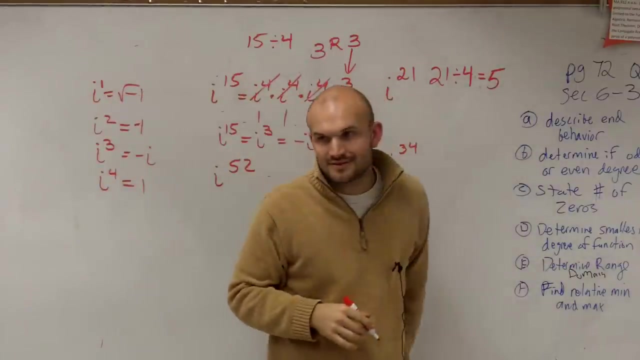 Rather than doing I to the fourth, I to the fourth, I to the fourth, let's just do it. Twenty-one divided by four is what. Twenty-one divided by four is what. Twenty-one divided by four is five. With a remainder of what Of one? 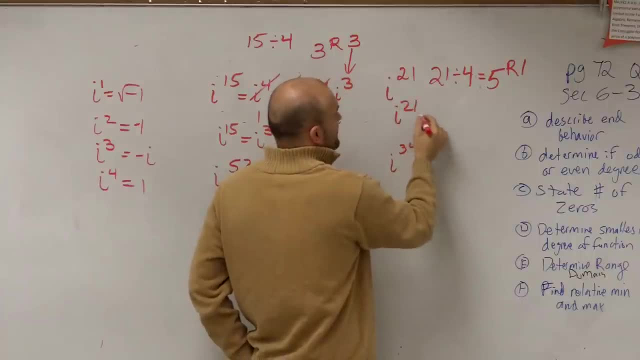 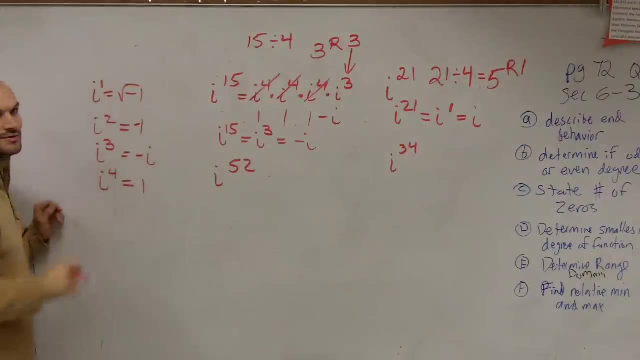 Twenty-one. So therefore, I to the twenty-first is the same thing as I to the first, which is equal to I. I to the first power is equal to I. Is everything equal to I in one? Well, unless it has a remainder of three, then it's I to the negative, I. Okay. Then we're going to look at I to the fifty-second. So all you guys need to do is take fifty-two, divide it by four. 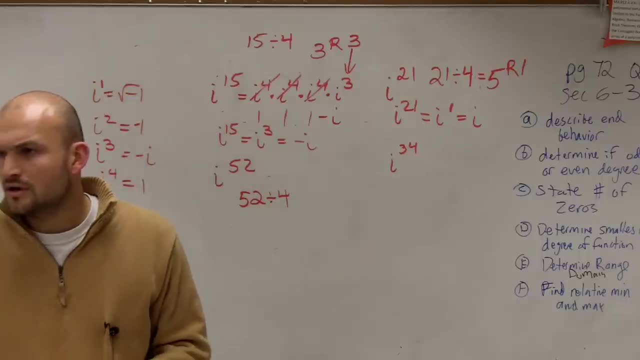 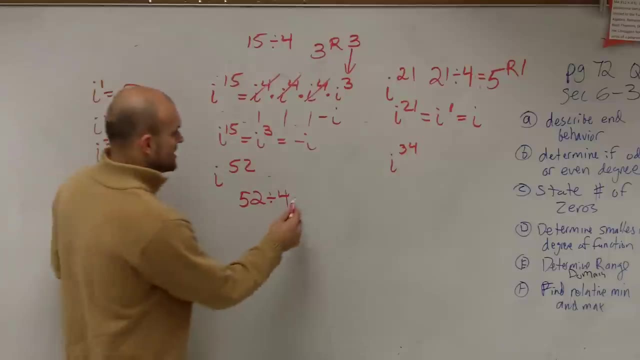 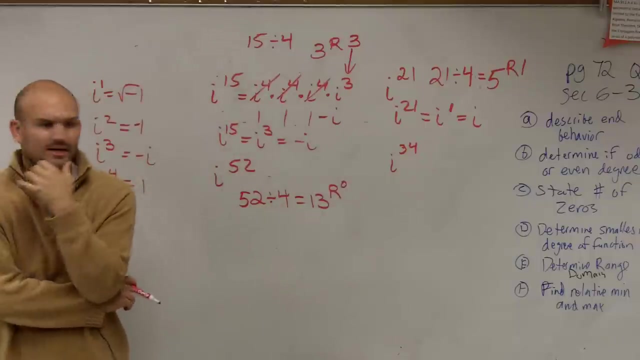 So how many times does fifty-two, Fifty-two, Fifty-two, Thirteen, Thirteen times? What's the? is there a remainder? There's no remainder, There's no remainder. So you could say it equals thirteen with a remainder of zero. Now this is where it gets a little difficult, because so far we had one, two, three, and then we go to four, and then we go back and repeat. So where is the remainder of zero? 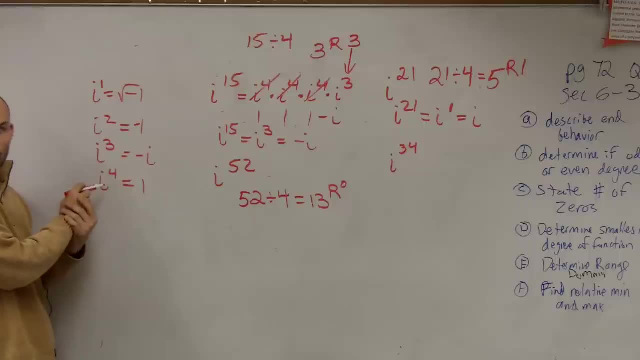 Well, ladies and gentlemen, if you divide something evenly by four, Four divides evenly into it, right? So that means that four is the same thing as really a remainder of zero. So what this is, then I to the fifty-second is the same thing as I to the fourth, which is equal to positive one.